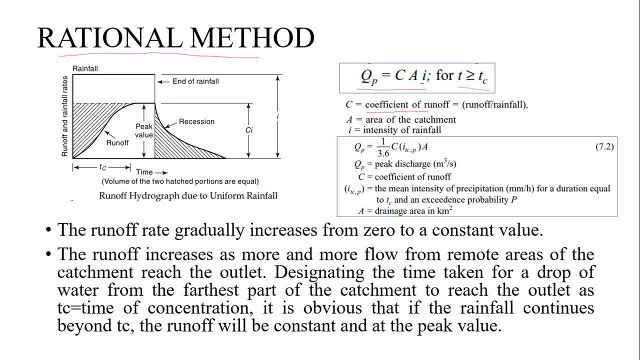 Tc. Now let us understand what is Tc. Tc is the time of concentration. Okay, So this is the flood hydrograph shown to you. This is the time period of the rainfall. Here the rainfall ends And here the recession occurs. Okay, Tc is the time of concentration when. 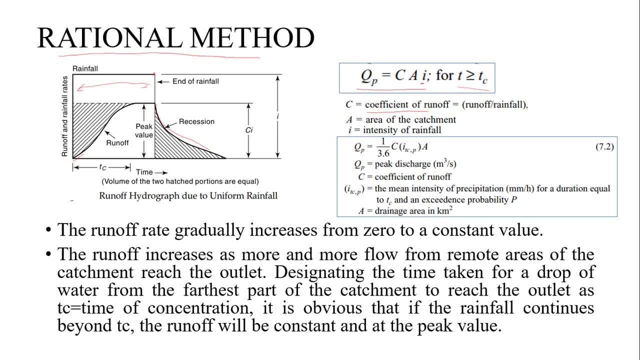 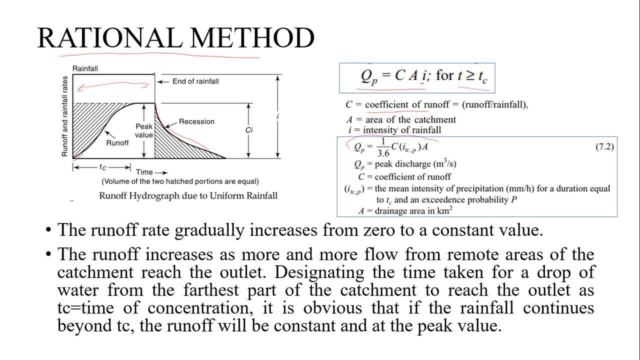 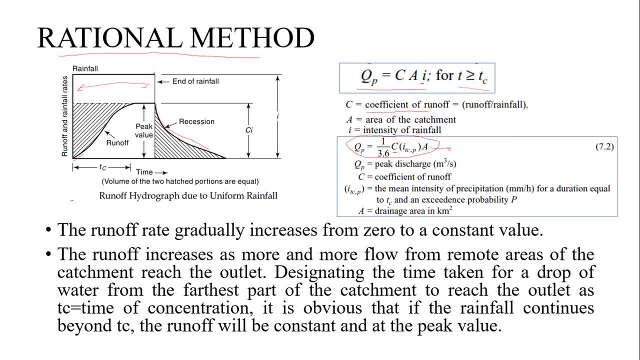 square. The C is same, But I is in millimeter per hour. Usually we use millimeter per day, but here it's used hour, So the factor 3.6 comes in the denominator. Otherwise it's a common formula. QP equals to CIA. Now let's see what are the methods for calculating. 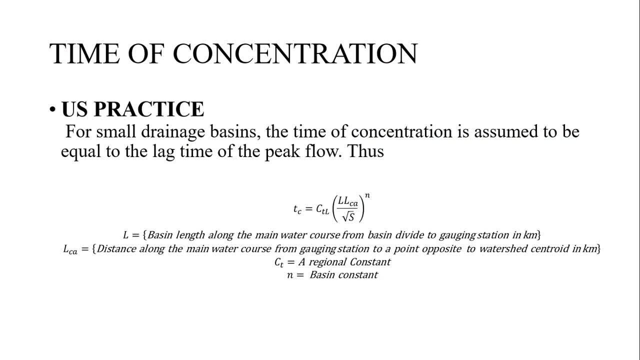 the time of concentration. so in the us practice formula this: ctl is a constant, n is a constant. these are the basin and the region constants. now, s is of course the slope, okay, and l is the length of the channel. this is basin length along the main water course, from basin divide to gauging. 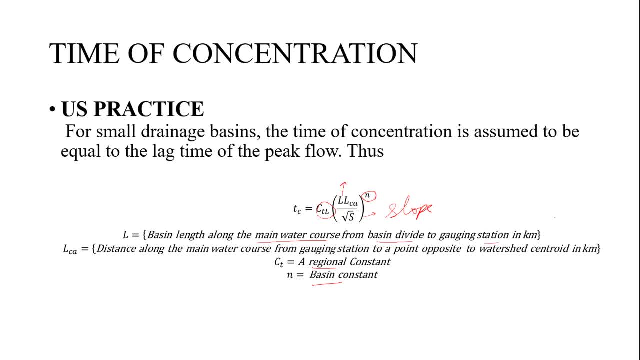 station. okay, so let's understand this with the figure here. so let's say this is my catchment, okay, now in this catchment, if, if, let's say this is my, these are the streams. okay, so what l means here is l is the distance measured along this line, this main channel, up till the end point. so, from this point to this point, along the 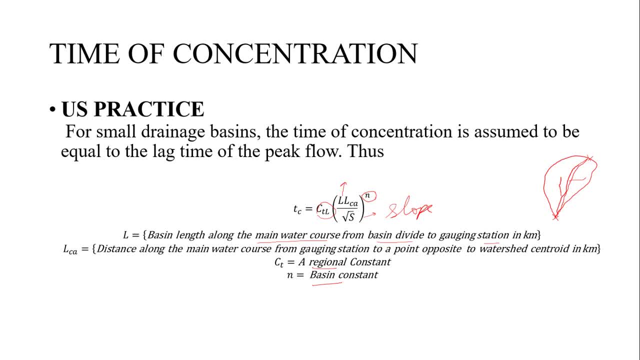 main channel. now what is the distance measured? lc? lc is the distance along the main water course. it's the same: the main water course, from gauging station- again, this is my gauging station- to a point opposite to the watershed centroid in kilometers. so what we do is we find the watershed centroid. let's say this is the. 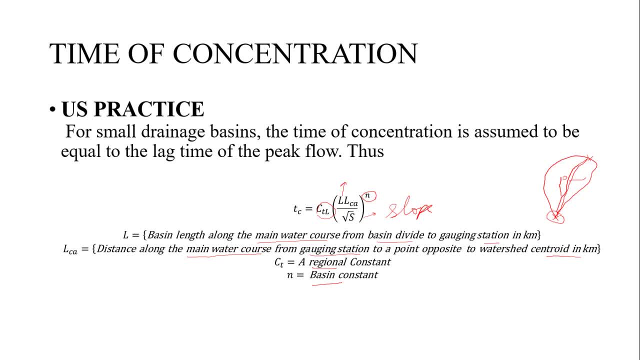 centroid here. okay, sorry, this is the centroid here. now the point will be on the main water course, so let me let me draw it again here, okay. so let's say let me draw it here, okay. so. so let's say the centroid lies here. so let's say centroid lies here. so my point would be here. 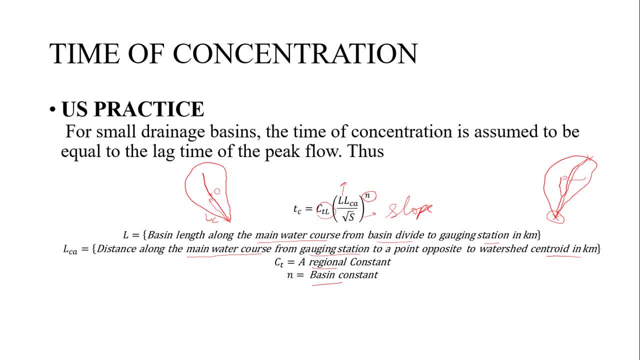 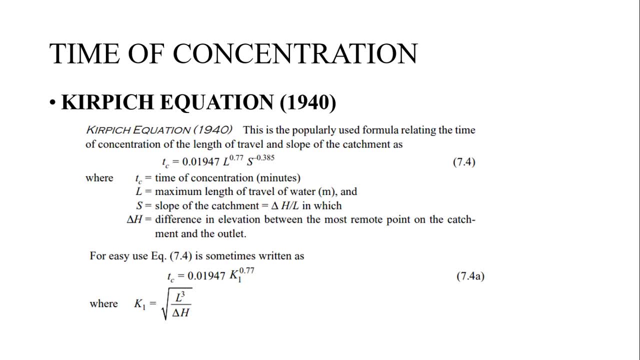 so this will be my lc and this entire length will be length l. i hope it's clear to you. so that's how you can measure the time of concentration. now there are some empirical equations, like kriplich equation. so in 1940 kriplich gave this equation which depends on l. again, l is the same, the maximum. 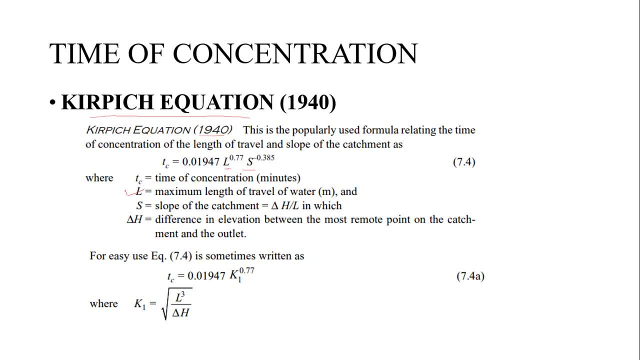 length of travel. s is a slope. there is nothing fancy here, so s is a slope for the catchment. this is delta h by l. now this tc, the same equation, has been rewritten in this form. so there is nothing but a simple calculation where you substitute this delta h by l from s. so if you substitute delta h by l instead of s and 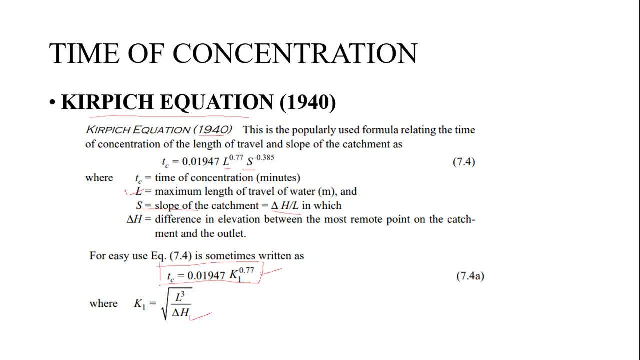 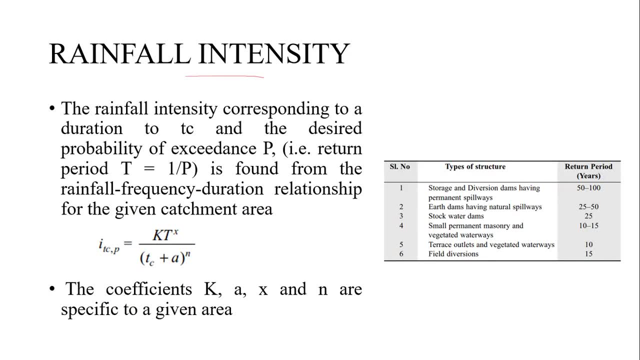 you simplify this, you get this equation where k? is this? so just a simple algebraic equation. now, what is rainfall intensity? how do you calculate this ic that we call the ic? it's a, it's a rainfall intensity. what we measure is corresponding to a duration, tc. you know. so we always measure for the duration tc, you know, and the 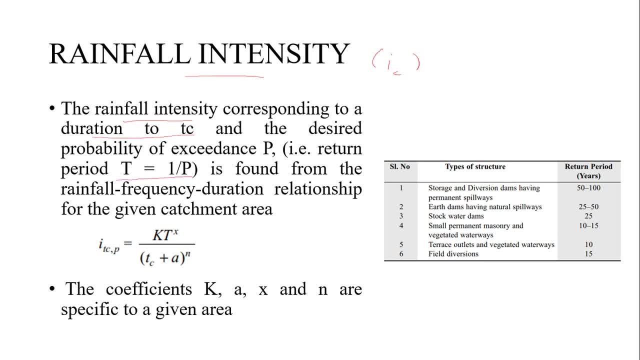 desired probability of accidents. t is equals to 1 by p. we always take the return p at the same, and this we can found from. we can find from the rainfall frequency duration relationship, you know. so this formula is given. so this, these all are constants. k is a. 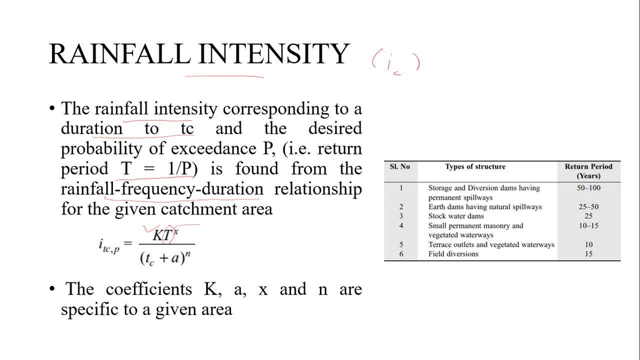 constant. you know. t is the required return period, x is a constant, tc is the time of concentration, a is again a constant, n is a constant. so these are the constant for a basin area. you know now when we're designing any structure. so let's say we're designing a dam. you know so. dams have 50 to 100 year return. 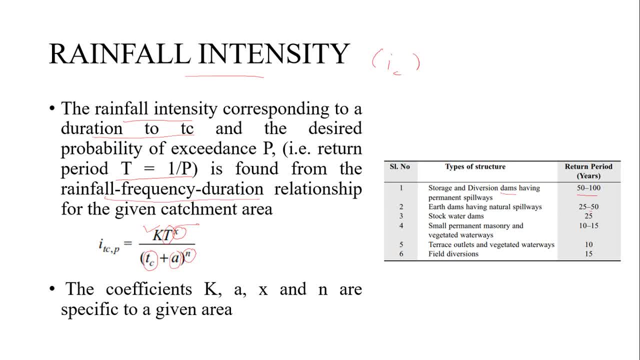 period. you know these are 25 to 50s for earthen dams. you know, for small outlets with vegetated waterways we have lesser time period. we do not worry about those, you know. so for dams we mostly worry, so that's why we keep it. 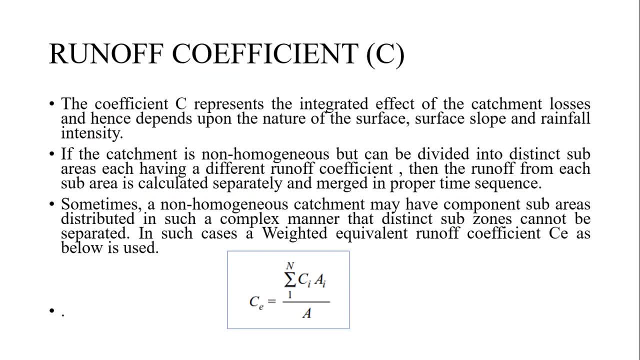 little bit high. now, what is the runoff coefficient? as I told, when we measured the peak flow it was c i a. so the c is the runoff coefficient- how much runoff is being generated from that particular area? so nothing fancy here. so this is, let's say, an average runoff coefficient you want to estimate? so let's. 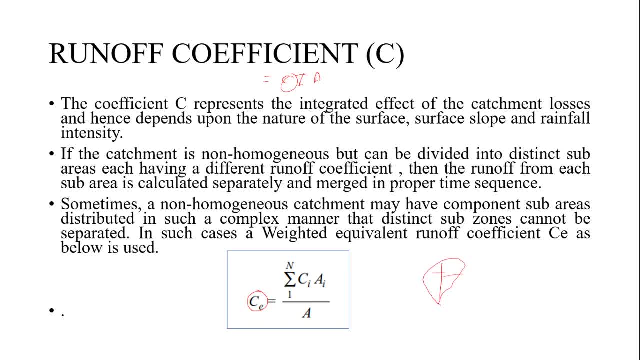 say there is a basin here and there are area one, area two, area three, area four. four areas are there, each having c, c1, c2, c3 and c4 as their runoff coefficient. so average runoff coefficient that you can find is c1, a1 plus c2, a2 plus and so on, divided by a1 plus a2 plus up to one. 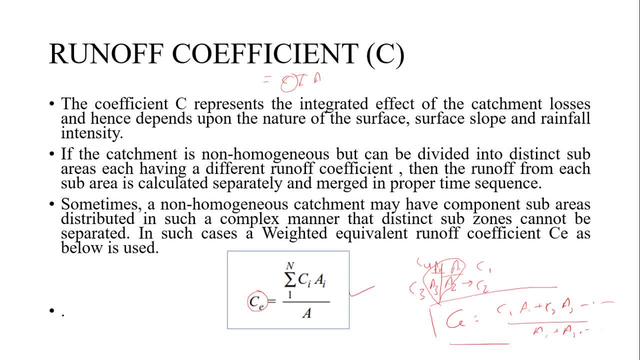 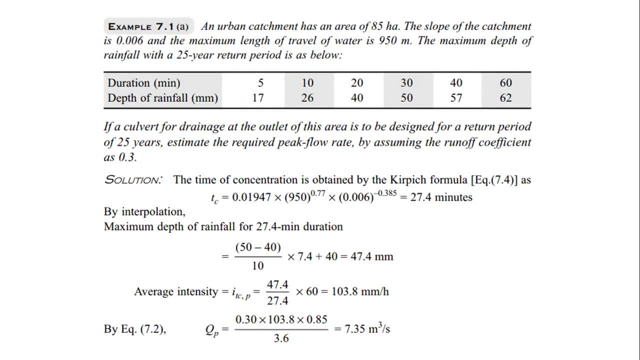 so. so using this formula, you can calculate the runoff coefficient. it is the weighted equivalent runoff coefficient. now let's take an example here. so we have an urban catchment having an area of 85 hectare. the slope is 0.006 and the length of travel of water- this is L- is 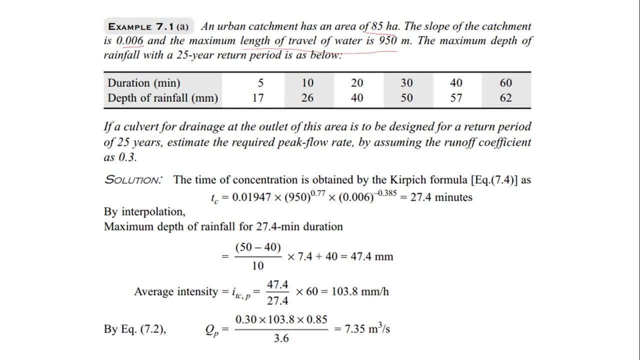 given as 950 and the maximum depth of rainfall for a written period, 25 written period is given. so this is the depth of the rainfall: 17, 26, 40 is your own- in mm. so as the time increases, duration increases, we see that the rain. rainfall is increasing. now what we want to find first of all, so the 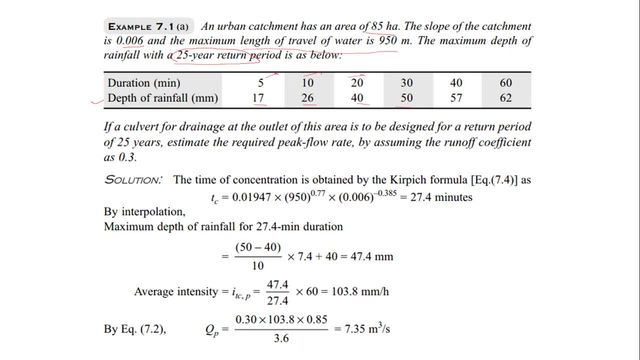 question is: we have to design a culvert for return period of 25 years and we have to estimate the peak flow rate, that is, Q peak. we have to estimate the runoff coefficient is given to us, right? so these all data are given to us. so let's. 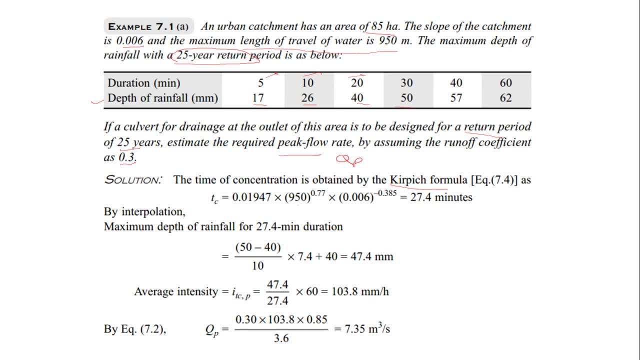 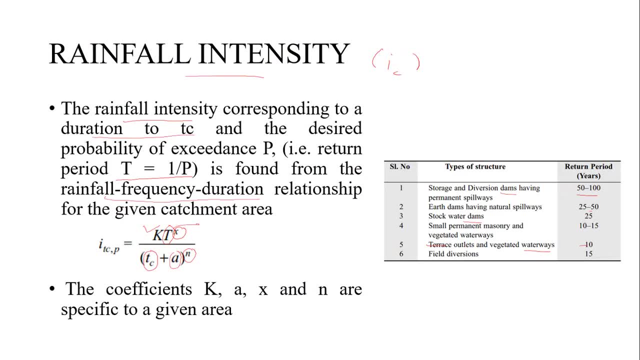 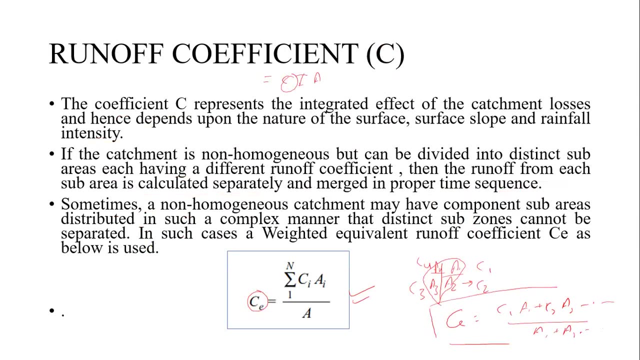 apply the Kirpich formula. that requires the area that we know and the slope s. so, using the area and the slope, let me show you again the Kirpich formula. so this was length of the channel- sorry, length of the channel and the slope. so we have put the length of the channel 950 and the slope 0.006, so we get 27.4. 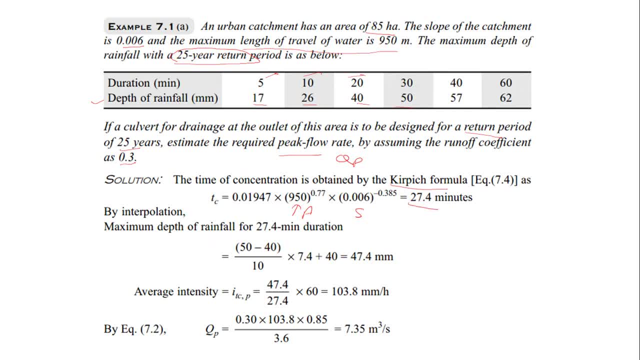 minutes as the time of concentration. now for this time of concentration, we know that the depth will be in between these. so we find the depth for a point 27.4 minutes. so we apply this formula: 50 minus 40 divided by 10. of course you know, simple in. 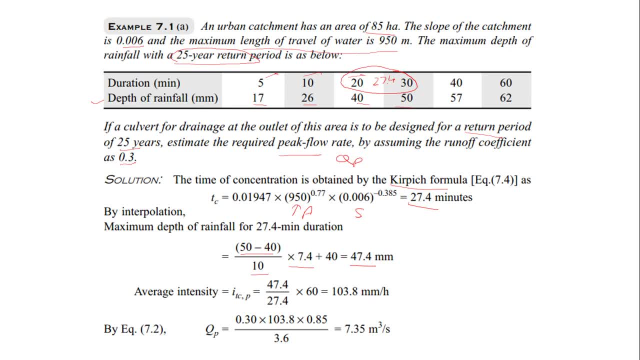 interpolation thing. so 47.4 is what we get here as the interpolated rainfall depth. now what is the average intensity? this 47.4 is the depth accumulated over a period of 27.4 minutes. so the average depth that we get is 103.8 after applying. 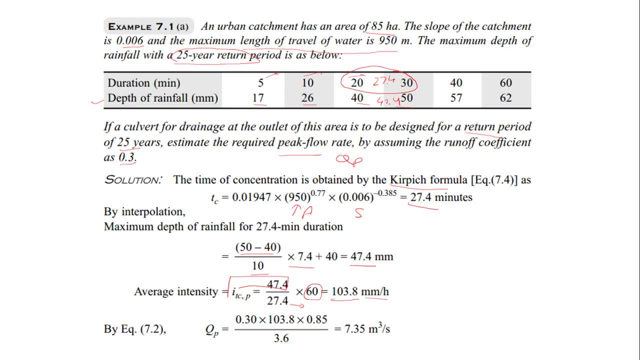 a factor of 60 that gives the value in millimeter per hour, of course, and using the formula CI, the average depth, area, and so area is given as 0, 85 hectares. so if you convert the area in kilometers square it becomes 0.85, and divided by 3.6 is the. the correction factor, the unit correction. 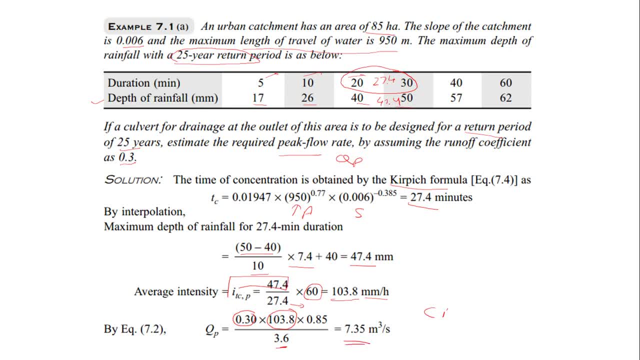 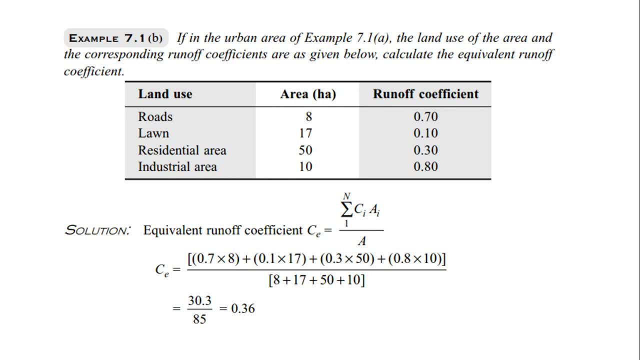 factor. so that's how you get the UPS 7.35 meter cube per second. now let's take another example here you are given with the different land use types: roads, lawn, residential area, industrial area- different areas are given and they run off. coefficients are given, so we just have to find the equivalent turnoff. 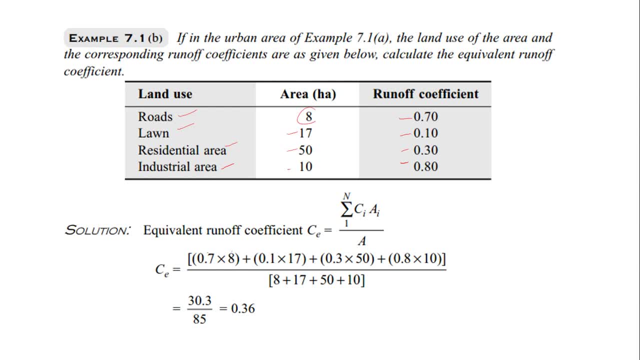 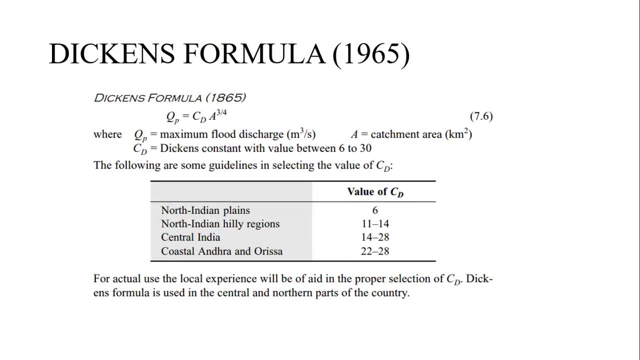 coefficient is a simple c1, a1 plus c2, a2 plus c3, a3 and so on. so you get the turnoff coefficient as 0.36. you can try that now for the peak discharge. there are some empirical formula also, so we use the runoff coefficient method rational. 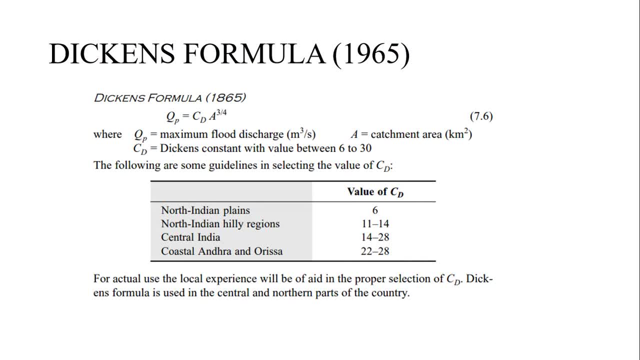 formula, and now we will see some empirical formulas. so this CD is the Dickens constant and that varies between 6 to 30. so for different regions the CD value is given. now area is of course the catchment area in kilometer square. you simply put the catchment area, you will get the peak discharge for that. 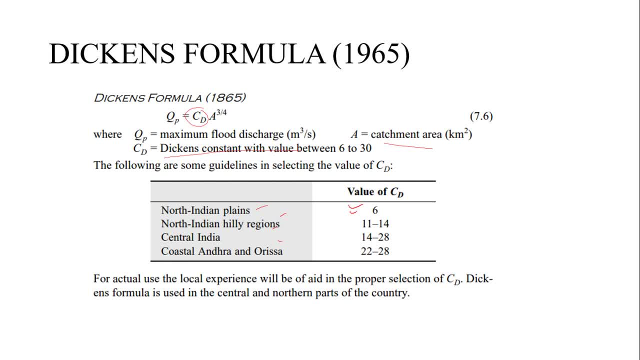 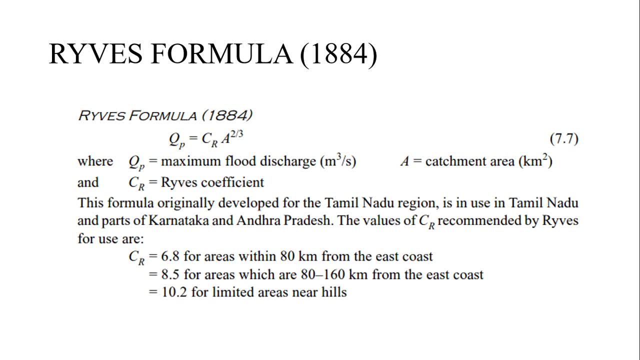 particular basis, so that basin has to be located in this particular regions. similarly, drivers also. I think we have discussed these things before. also now, CR is the drivers constant. so this is 6.8 for areas within 80 kilometer from the east coast. like that, as it goes far it becomes 8.5 for areas near hills. so these are mostly for. 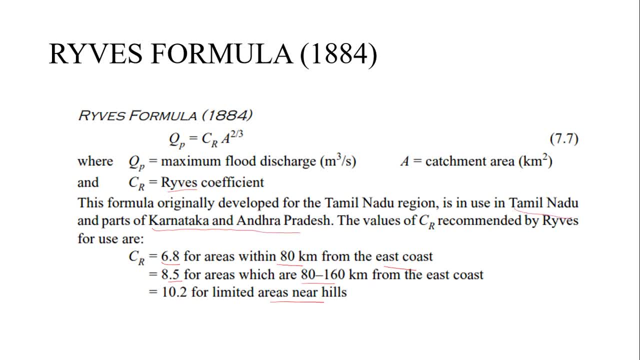 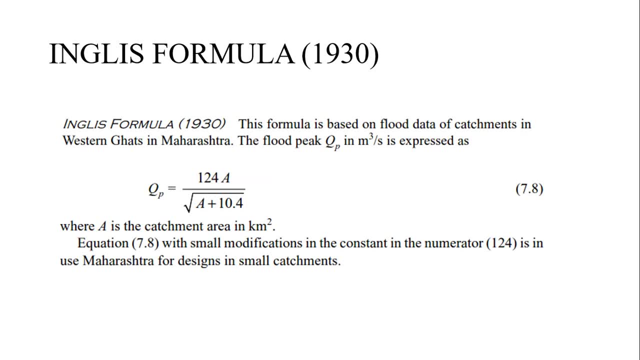 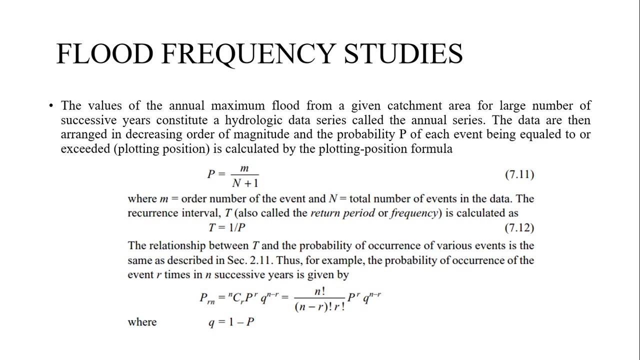 the Karnataka and the produce Tamil Nadu, right. so that's how you can find the QP decrypt and thatoperation is all right. so what's left is the deltas efficient state. subject: APA cases. and in sunset inspired that study, the decision making of the Metallic ре. 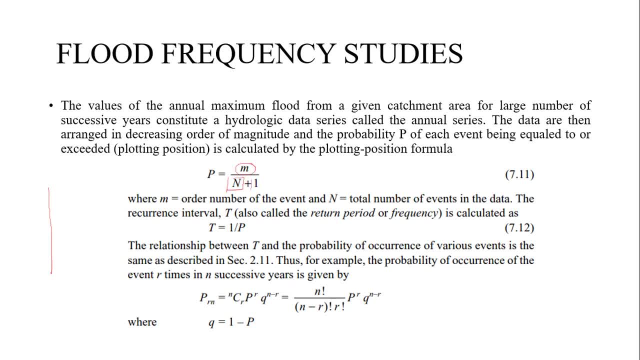 position divided by n is a total number of years plus one and is a number of events in the data. M is the order at which it's occurring and of course, the inverse of this, P, will be your time period. so once you get the probability of occurrence, you can of course get the probability of occurrence R times in n. 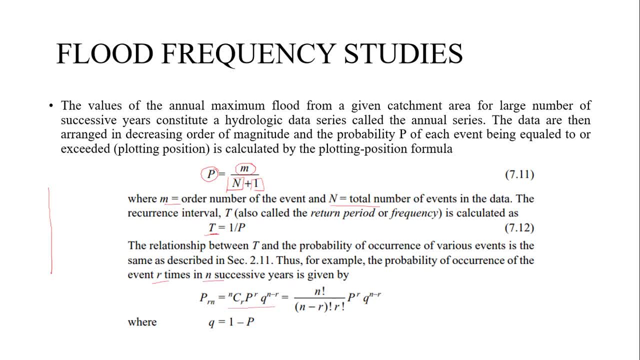 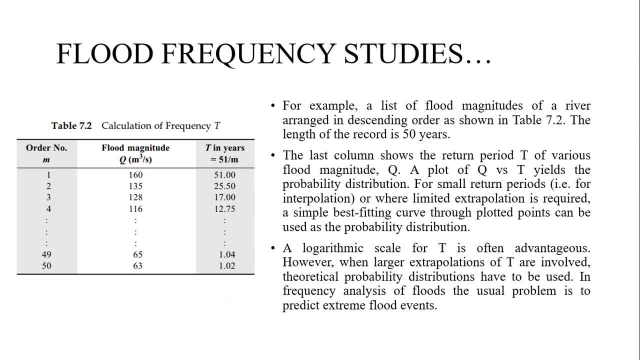 successive years. that is simple by the binomial formula NCR, PR, Q, n minus R. so this you can do here now. for an example, the floods have been arranged: 161, 35, 128, 116, like that, 50 years of flood has been arranged. so the return period for this 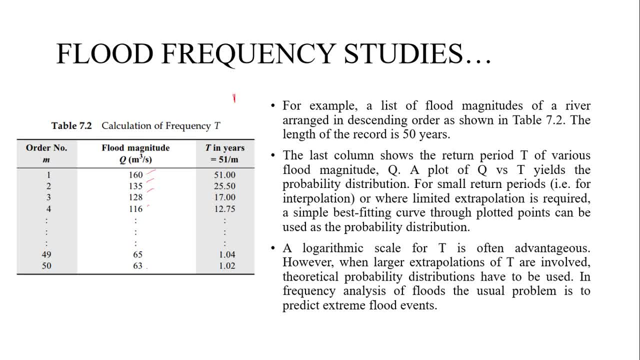 first case would be: first position divided by 51- this is the probability- and the time period will be 1 by P, that is 51. so it's a simple calculation you can do and that's how you can arrange them. and then what we do is you plot. 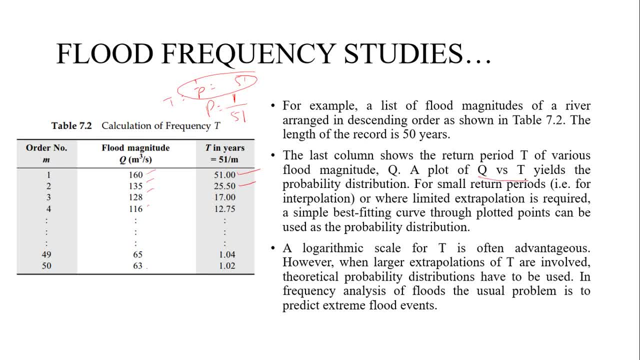 the time period and then you plot the time period and then you plot the time period and then you plot a curve of discharge versus time. so you plot a curve so how the discharge varies with the return period. and so let's say you got this discharge in the time period and you can. what you can do is you can fit a curve. 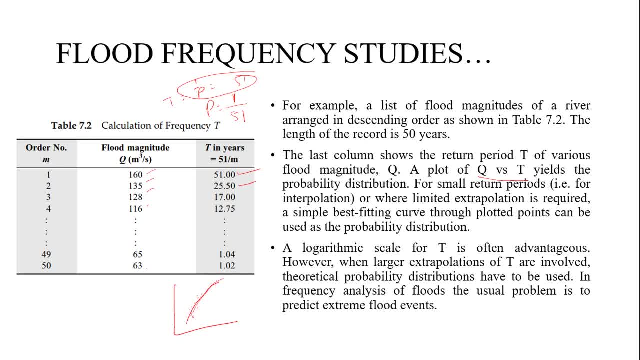 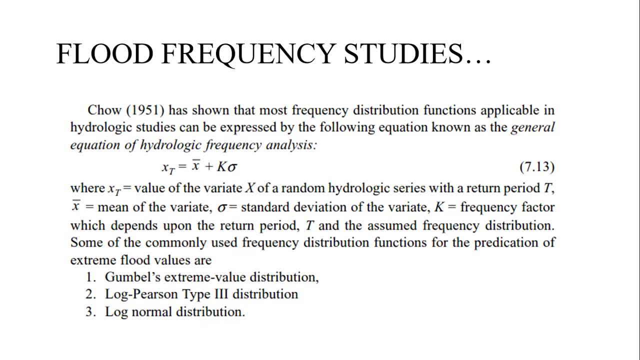 and using this curve you can estimate the peak flood for any given return period. so this is called the flood frequency studies and there are number of formulas given for that. so Chou in 1951 has shown that the frequency distribution function follows this equation. XT is X bar plus K. Sigma XT is any variate for our case. 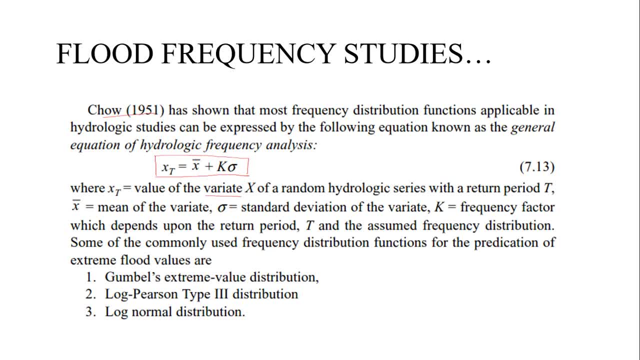 it's a discharge for the return period, T will be the mean discharge or the mean variate plus stand deviation of the data- in our case it's a stand deviation of the discharges- and K is any frequency factor. this K can be anything that depends on. 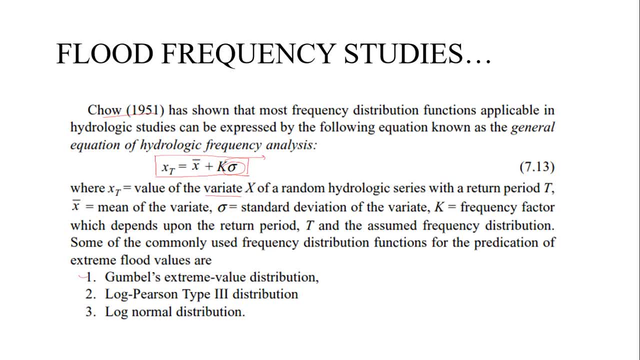 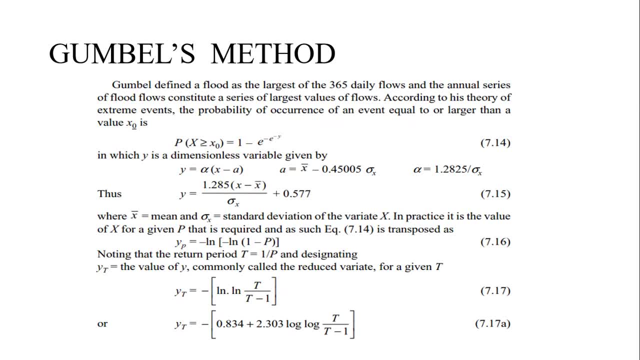 the number of distribution that we are using. it can be gumbel, log Pearson, type three or log normal. whatever distribution we are using, this case different. now let's see the gumbel's distribution. so gumbel distribution says that probability of occurrence of any 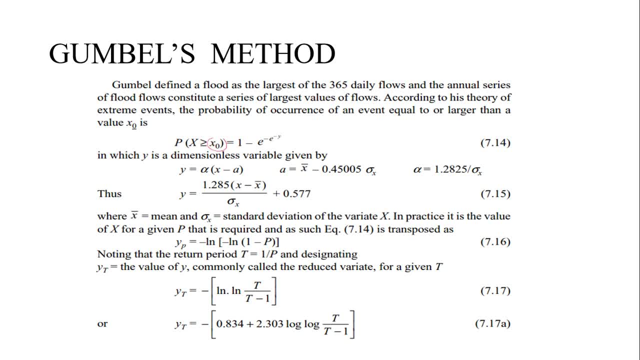 event equal to or greater than X 0. X 0 is the is any particular value that you have chosen? is 1 minus exponential to the power of, minus exponential to the power minus one. this is a equation that gumbel. give probability now in this. 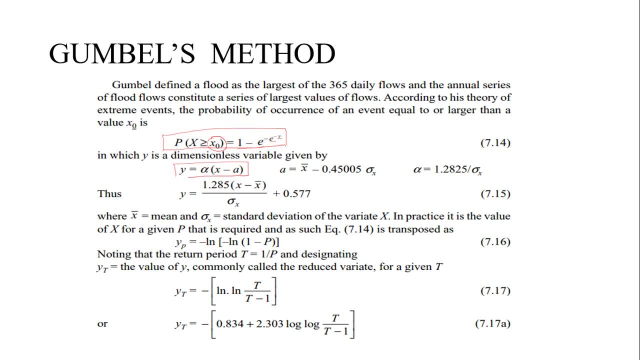 equation y is given by an alpha times X minus a, where A is X bar minus 0.4500, 5 Sigma X and alpha is 1, 0.2825 by Sigma X. so when you combine all this equation, or the only variable in this equation is Y. so from this equation we get Y is equals to. in these three equations we get Y equals to one point to eight, five X. if the 2 basic things we get are 1.18, 도1825, X and 1.2825, come to that state: 1.都有 로2 에이 24286. 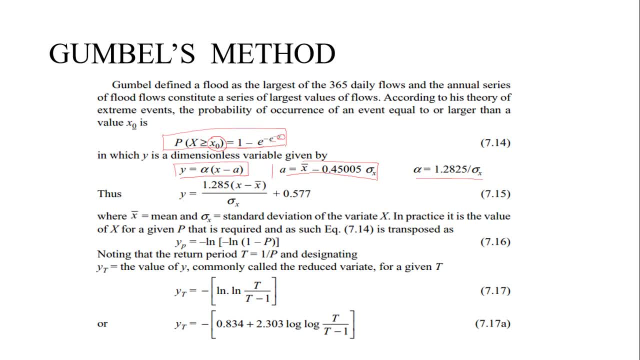 minus x bar and you can do a simple calculation upon sigma x plus 0.577. this equation is for infinite number of data sets. remember that, and i will use it for a lesser number of data sets also. so x bar is your mean, sigma x your standard deviation. so this is mostly known. x bar is: 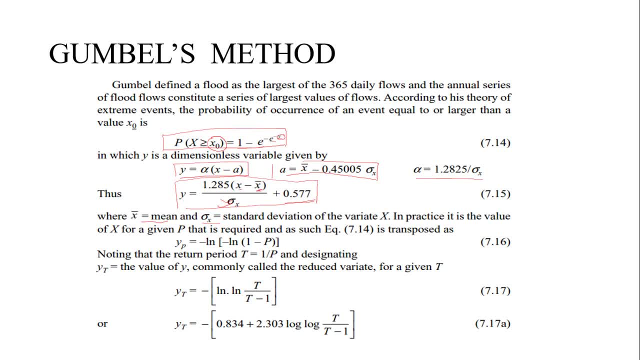 mostly known, and x is the variable and of course y is the another variable. now, if you see this equation 7.14 and you rearrange this equation, you will get some equation. for the y p is equals to minus log, minus log 1 minus p. this can be done easily, right, just by changing the sides and all. 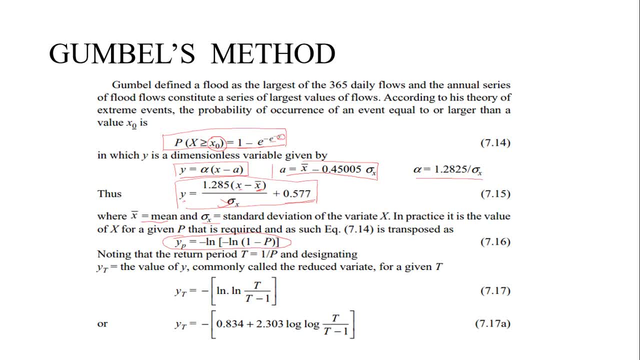 now this y p for a probability, so you can change p to t, of course, because p is equals to 1 by t, so this y t will become minus log, minus log t by t minus 1. you can do a simple calculation, and now this can also be converted to log base 10 and you will get some constants here also. 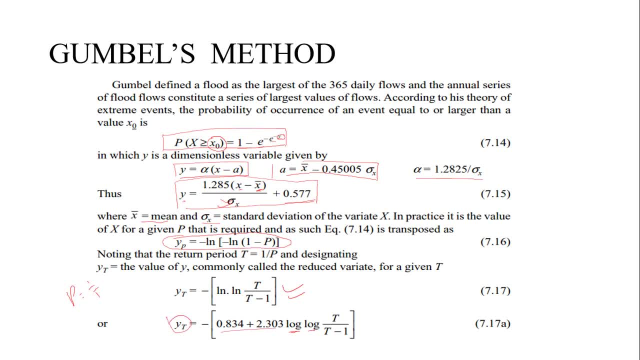 that's why you got this equation. so y t for a given return period you can get from here, so this y t can be known. so are you getting the equation here? see: y is 1.285 x minus x bar over sigma x plus 0.577. this x bar will be mostly. 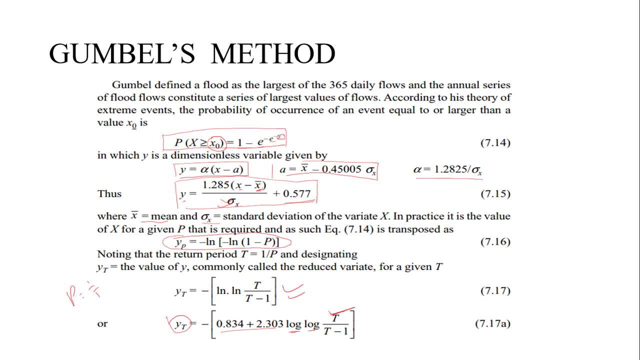 known sigma x will be known. this y can be calculated for a given time period, t from this equation or from this equation. so from there you can get the x t, that is, for that particular return period you can get the x t. see here now this equation. if you see, if you realize this, 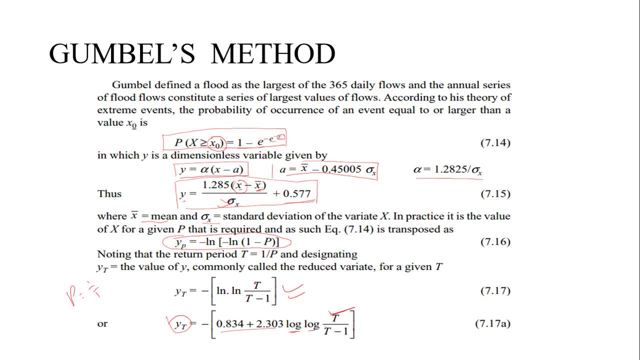 equation. what do you get? let me realize this equation. you get y sigma x, you know. so that will be equals to 1.285 into x minus x bar, you know, and there will be some constant. let's call it minus minus 0.577 plus. this equation equals to 1.285 x minus x bar. this looks something. 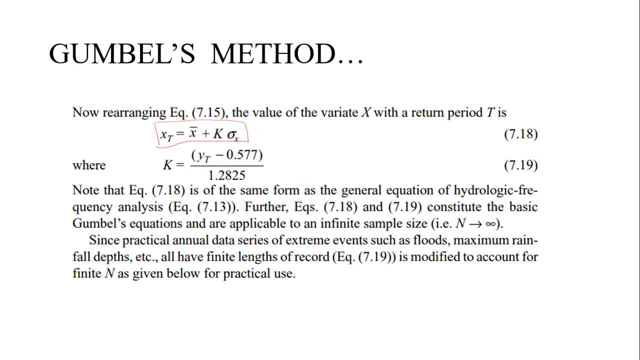 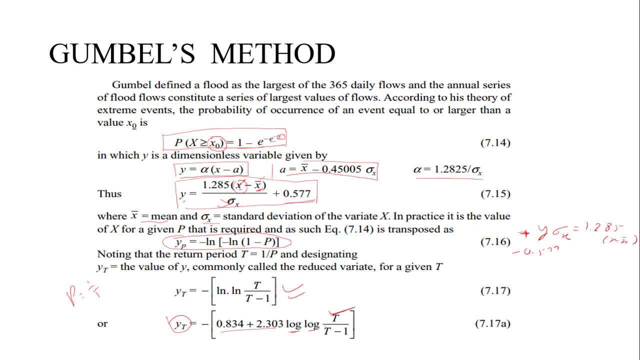 like this: right: x t equals to x bar plus k sigma x, because x and x t, this is x T, this is x bar, x T bar. Now the sigma x will come with y, sigma x will come with y and this k is a constant. 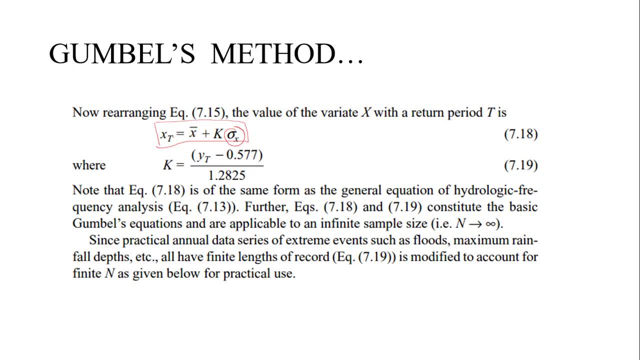 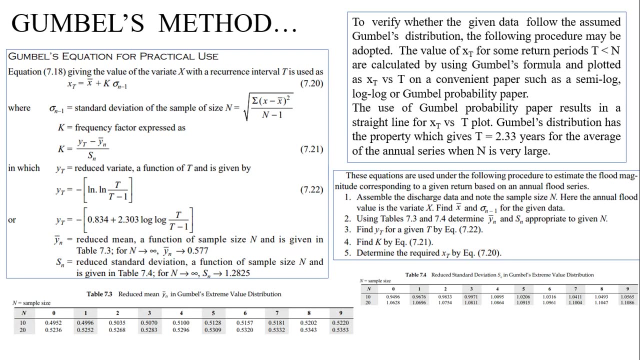 of course. So this k becomes yt minus 0.577 over 1.2825.. I hope this is clear. and this is applicable to an infinite sample size. Remember that. Now for the practical application, how we are going to apply that. Practical application means when the data is not infinite. 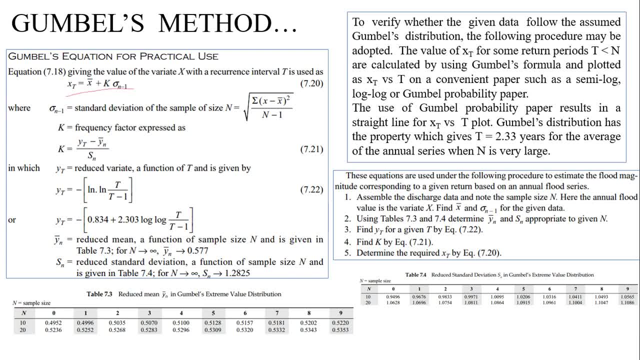 but it is finite. So xt is x bar plus k sigma n minus 1.. So stand division you can calculate from this equation. k is the frequency factor. We know this yt minus yn over sn. Now, instead of this 0.577, 1.2825, we are using this yn and sn. Now this yt can be calculated from: 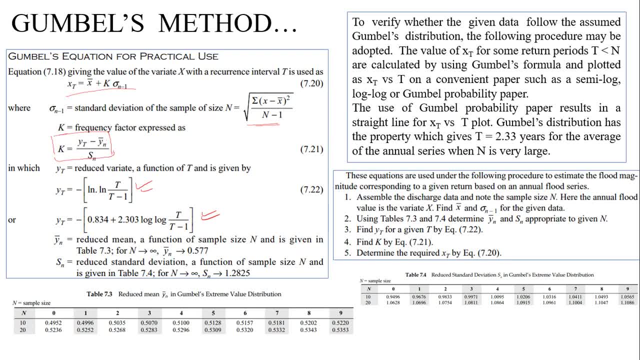 this equation or from this equation. So this is simply yt. you can calculate This yn, bar and sn. these you can calculate from this table. So let's see, Let's say some tables are given to us for different sample size. So this is the value. 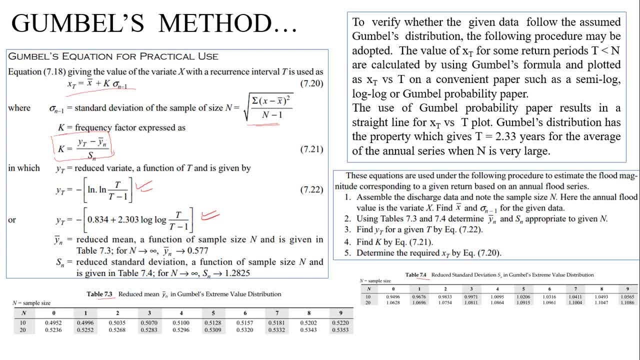 for yn. So you can see, as your sample size increases, this value reaches to 0.577 and here also, this value reaches to 1.2825 as the sample size increases. This is for the sn, Alright, So I hope this part is clear to you. Now this to check, if the data follows: 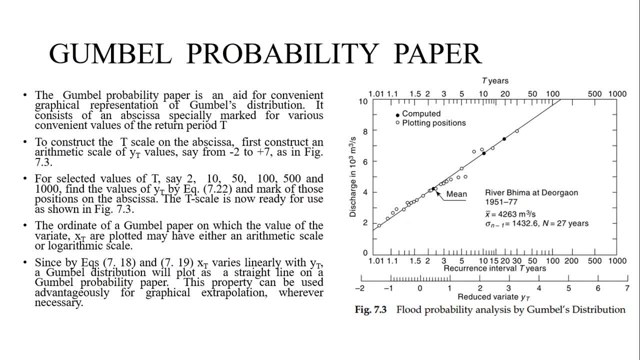 or not. we mostly use the Gumbel's distribution, Gumbel's probability paper. So on the x axis we have the reduced variate yt and on the y axis we have the discharge and definitely we will get a straight line equation. if you plot this data in terms of 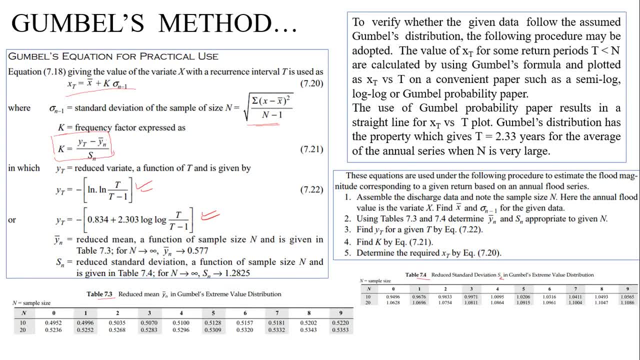 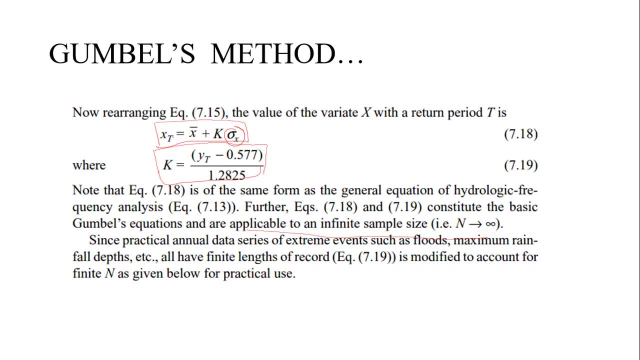 yt and qt. So you can see here this: here is the yt. So if you place this yt here, you will get xt is some constant plus yt. So this is straight line with yt. Now this is how you will see it. This is straight line with yt And here the frequency interval. So this: 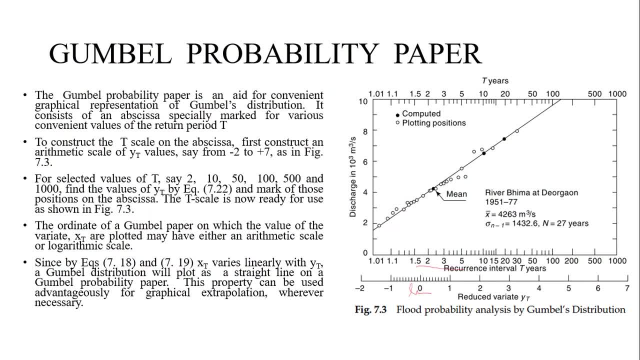 is the linear scale. You can see what the yt is. So this is the linear scale. This is the see here, and this is logarithmic scale, because yt has a logarithmic relationship with the written period. so that's how you'll get this logarithmic scale. so this is the written period. 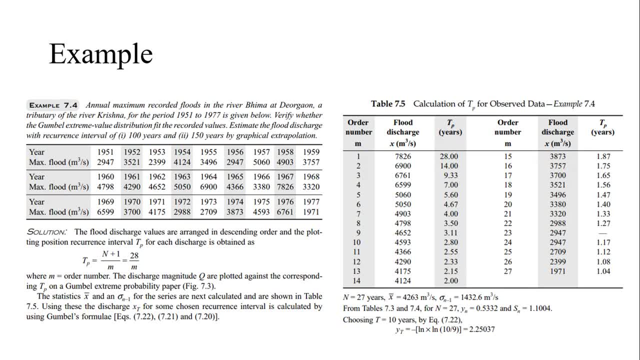 all, right, now let's take another example. so in this example we are given with the floods in some river and for the period is also given, we have to verify whether this follows the gumball extreme value distribution or not, and then we have to estimate the flood discharge for 100 year and 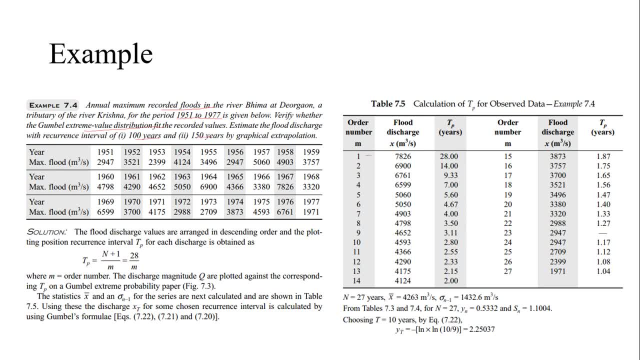 150 years. so what we do? we arrange the data one, two, three, four highest, two lowest, and for that we get the written period. of course it's a 28, 27 year data, so written period will be 28. then it goes on decreasing 14, 9.33 as a simple formula. i hope you know this is nothing but your n plus 1 by m, right. 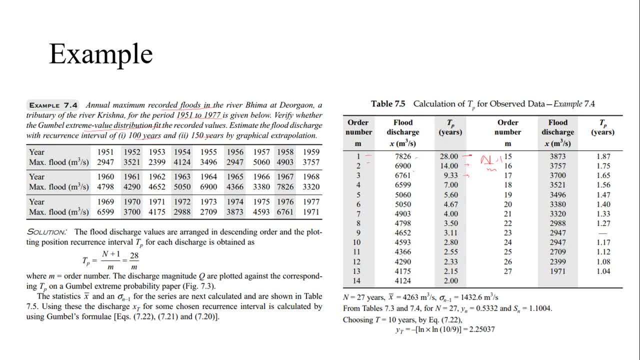 for m equals to 1, this becomes 28 because here- and it's 27 x bar- the mean of this data flood discharges is four to six, three. the stand deviation you can calculate now from the table: 7.3 and 7.44 n equals to 27. you can. 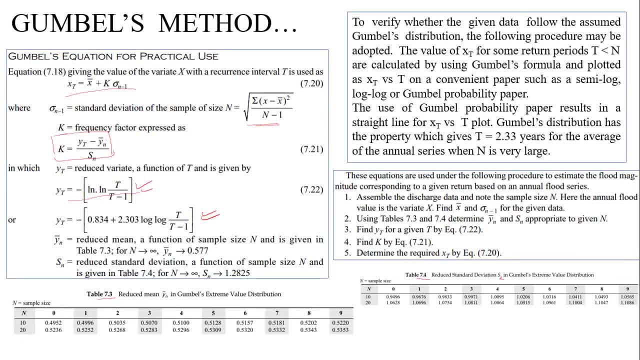 calculate this yn and sn and 27? i think i don't have it. yeah, i have it here. so 0.5332, 0.5332 is the yn, then you go for sn. 27 is one point one, one, one, zero, zero, four, one point one. uh, 27, one point. 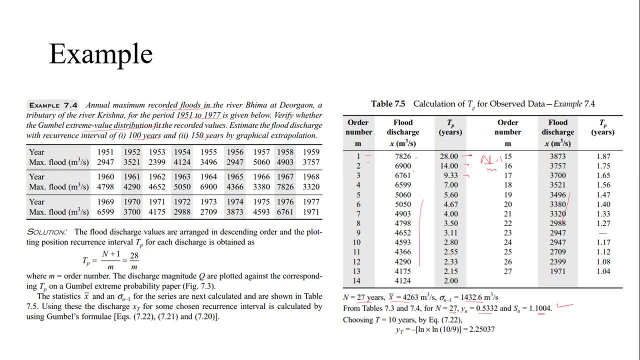 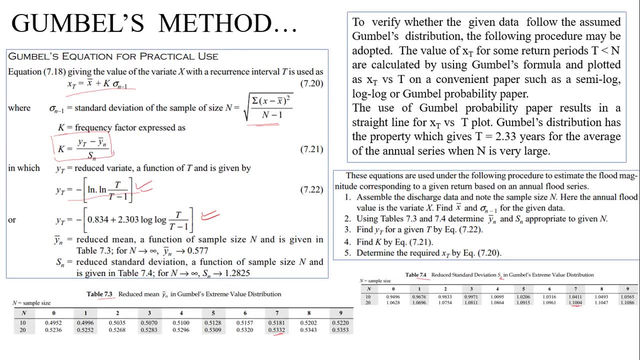 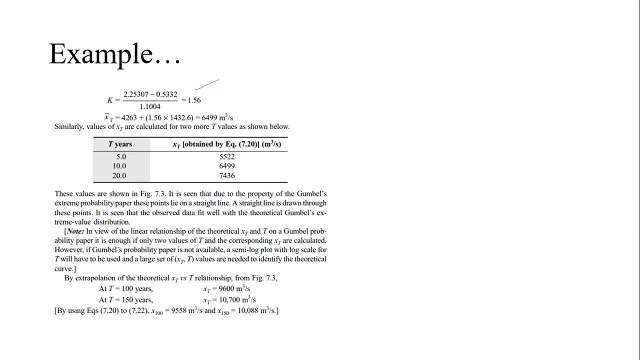 one zero zero four. so this we have used here. okay, so you can calculate the yt. uh, it comes out to be log log. you know. so this is log log, t by t minus one, this how you get the 2.250: 37. from that you can calculate the k value and then you can calculate the case formula. simple formula. 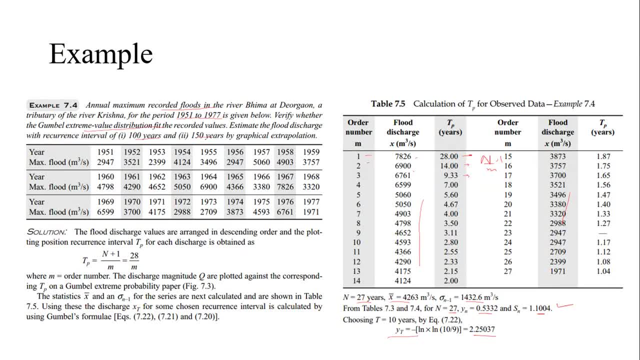 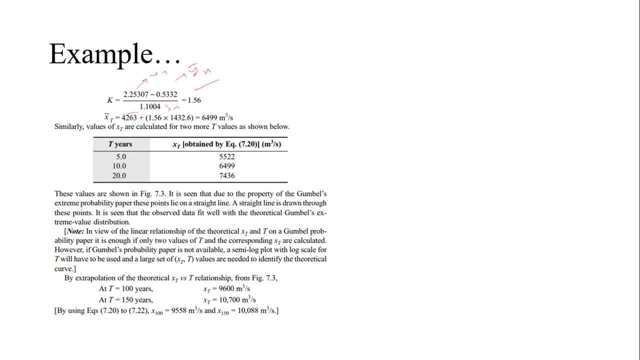 k is yt minus yn bar upon sn. this you can calculate: this is your yt, this is yn bar and this is your sn bar. and xt is nothing but the mean value x bar plus this k value that you just calculated. 1.56 x, this is 1.432. is your sigma n minus 1? right now, once you have calculated that, you can get the. 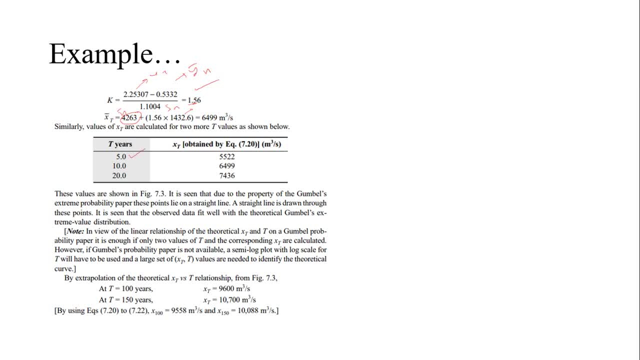 xt value for any written period. so this is: this is for the written period. how much you got for the 10 years. you can do it for the 20 years. you can do it for the five years, if it follows or not. what you can do is you can get the uh for different time periods, you can get the values of xt and. 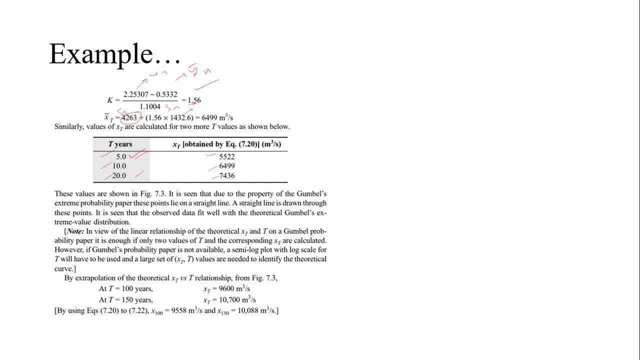 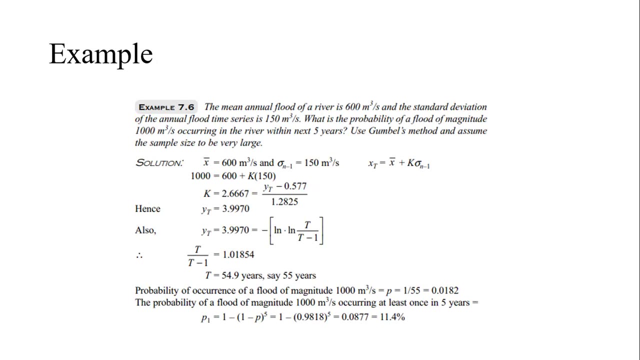 you can see if it follows the linear graph for yt versus xt. if it is linear, yes, it's a, it's follows the gumbel distribution. there's another example here. you know, in this example you are given, with the mean annual flood, 600 meter cube per second. so x bar is given to you, sigma n minus 1 also given to you, standard. 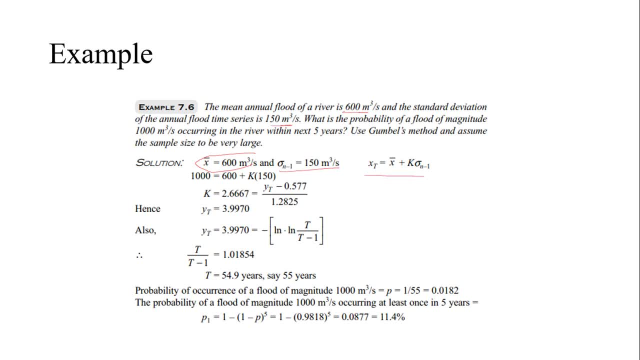 deviation xt. this equation we know very well. uh, we have to find the probability of flood: 1000 meter cube per second right. we have to estimate uh probability, actually that occurs within next five years. so we have to use the gumbel's method here again. so we are given with x bar, we are given with sigma right, we are given with this xt value. 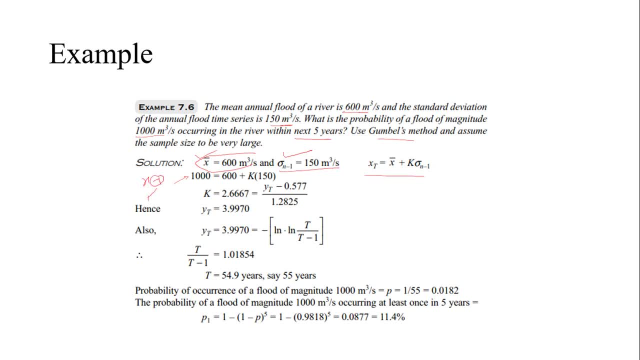 so we are already given with xt for t equals to five years. so if you apply this equation, uh, xt, this equation, xt equals to x, bar plus k, sigma n minus one. this is known to you, this is known to you, this is known to you, so you can calculate k. you got the k. two point six, six, seven. 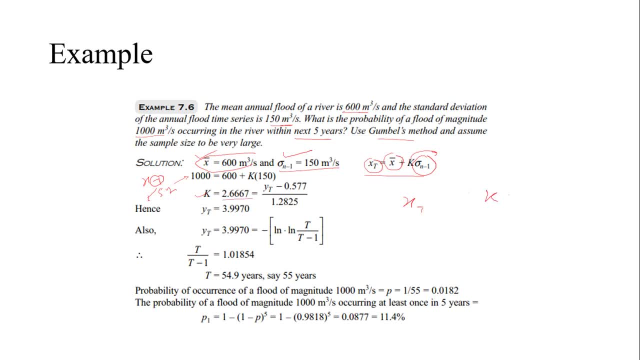 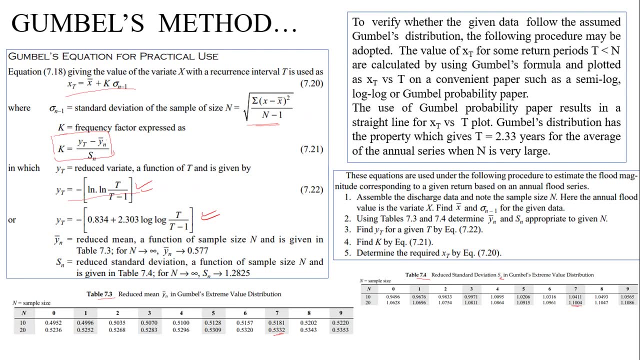 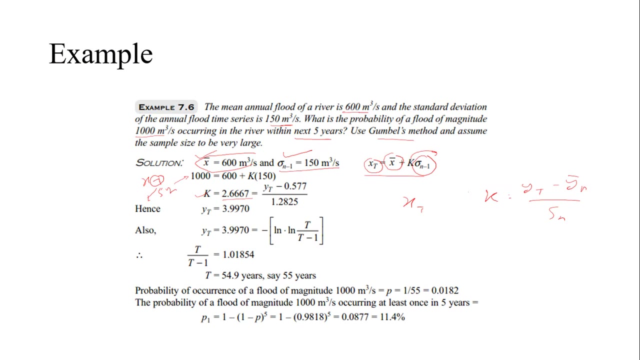 now this k. if you remember this k, it was yt minus yn bar over sn, right? you remember that this was yt minus yn bar upon sn. now, what is not known to you. so here it says: if you assume that the data follows sample to be large, so it's given sample size is very large. 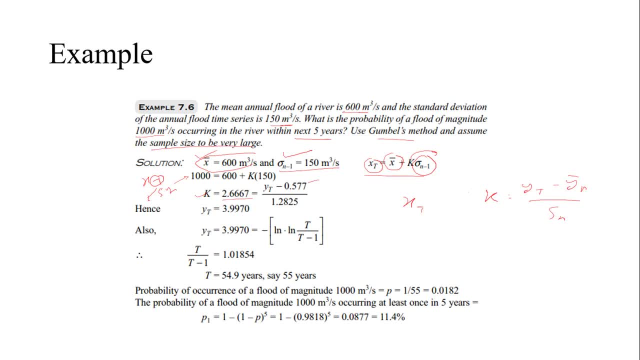 that's why this yn bar is point five, seven, seven and this sn is one. point two, eight, two, five. so from this equation you can calculate: the yt is a function of return period. so from this equation you can get the return period 55 years. so this XT, so this T was not 5 years, so T we calculated as the. 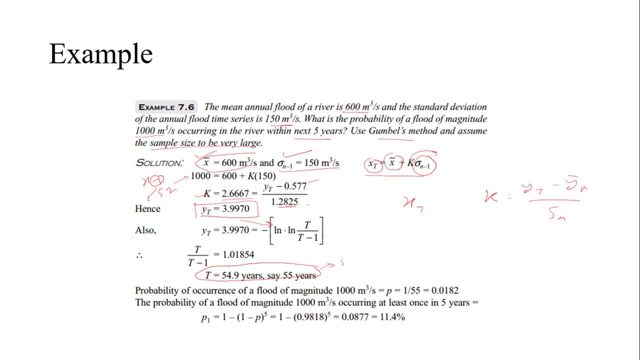 55 years now for this 55 years discharge. so discharge is 1000. now this 1000 meter cube per second has a written period of 55 years. so what is this probability? it's probably is 1 by 55, correct, so this is 0.0182. now 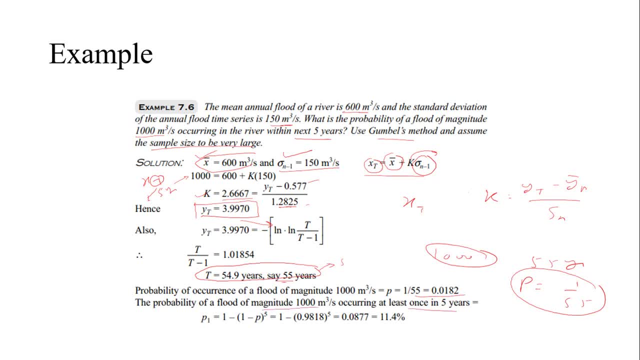 this flood, occurring at least once in five years, will be 1 minus Q raised to the power n, 1 minus Q raised to power n. so see Q raised power N means not occurring in first year, not occurring in second year, not occurring in third year, not. 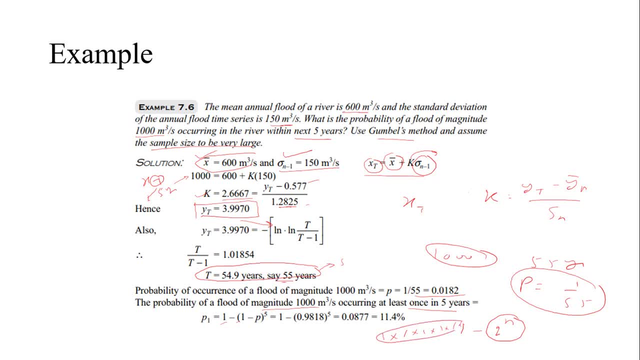 occurring in fourth, not occurring in fifth year. this makes it Q raised to the power of 5. if you remove this value from 1, that means it occurs at least once in 5 years. this means that water will not flow. otherwise occurs at least once in the next five years. So this is how you can calculate it Now. 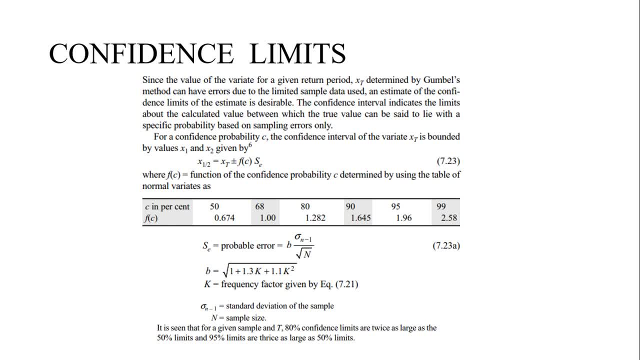 Chow also gives some confidence limits. So from the same equation you can get the confidence limit. So for any function we mostly for any data that we are predicting, we always apply confidence interval. It's upper limit and the lower limit by how much confident? 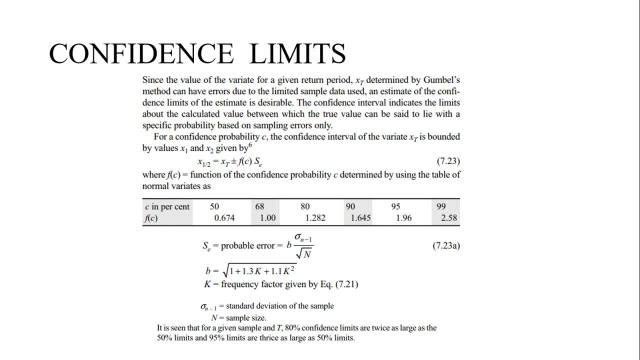 we are with the data, So it's a simple formula. So X was see Xt. you already know Xt was calculated. What we just have to do is, once we know this data, we just have to apply some plus minus to this data. That's how we calculate the confidence limits, right? So this formula? 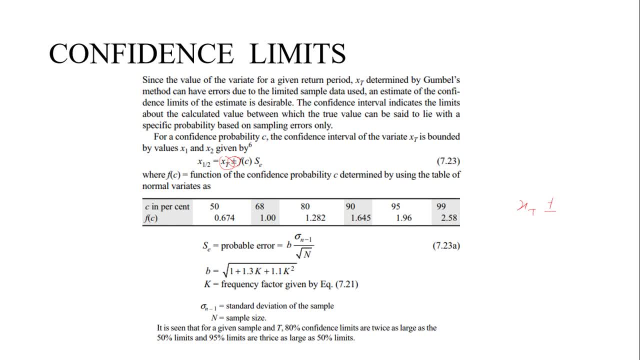 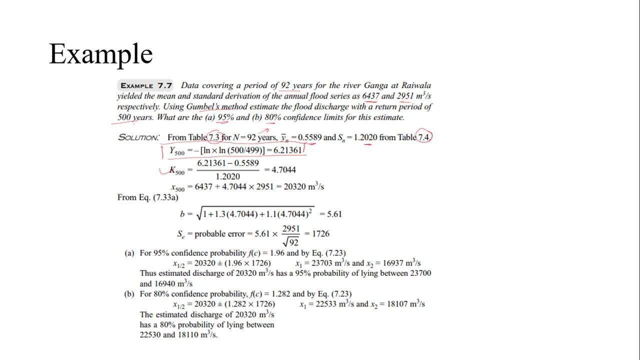 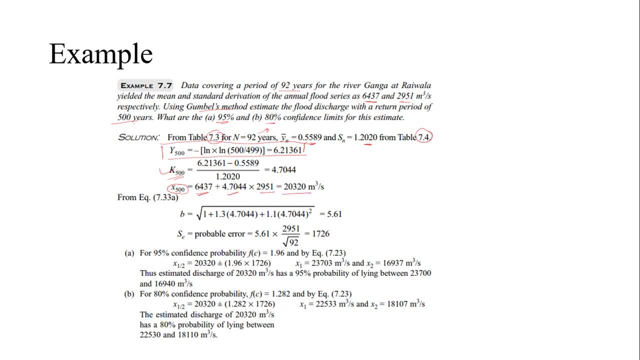 this comes out to be 20 320 meter cube per second. now you have to calculate the confidence limits. for that you first need the b value. this is 1 plus 1.3 k plus 1.1 k square. you get this value. then sc, of course, is the sc is b. you just calculate 5.61 b. this is the standard division. 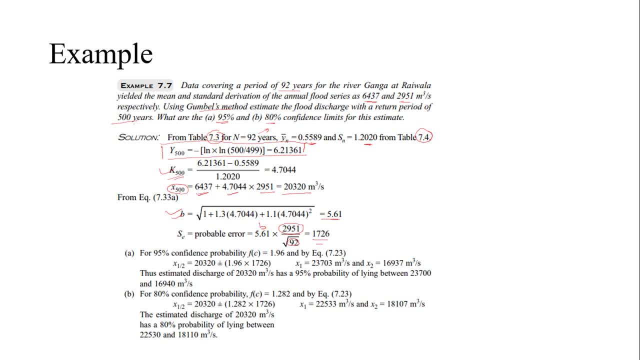 this is sample size root n. you get this sc now for 95 percent confidence interval. you have: fc is 1.96. so this is the mean value, 2320 plus minus 1.96. into what is the value se? you just calculated sc. the same thing goes. so one is the plus, one is the minus here. okay, it's a simple question. 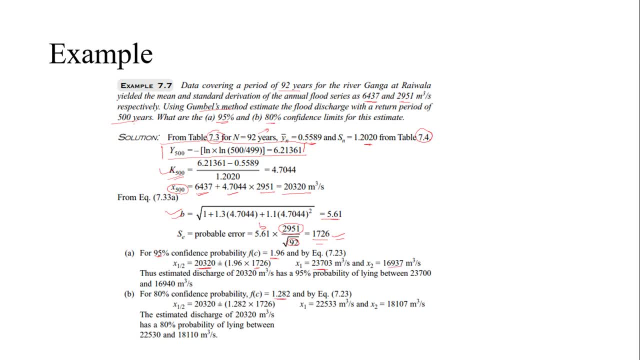 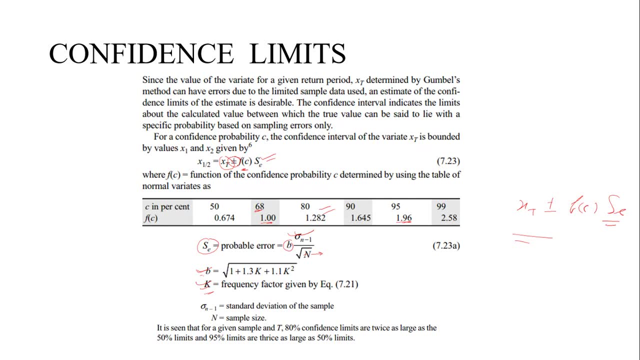 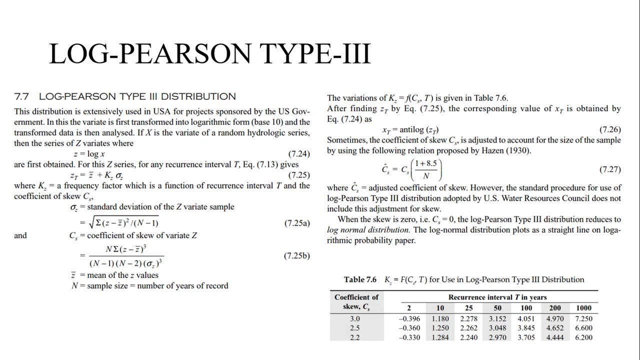 the same thing you can do with 80 percent, whereas you have fc is 1.282 for the 80 percent right. some major numbers you must remember. maybe this one and this one you can remember. others may be not required. so this is log p3 distribution. 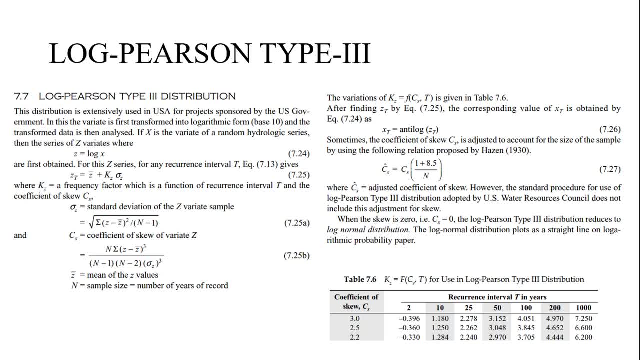 just like we have the gumball, we have this log p3 here. what we do is we convert the discharges in the logarithmic case, so z equals to log x and instead of xt- actual discharges, we deal in the terms of z plus k. so we convert the discharges in the logarithmic case, so z equals to log x and instead of xt actual discharges we deal in the terms of z plus. 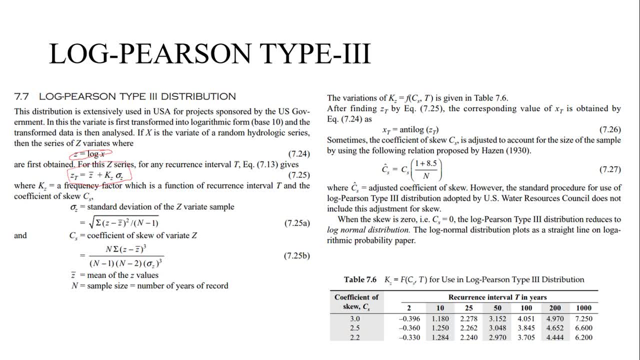 kz into sigma z right. so z bar is of course the mean, but in the logarithmic form. kz is again a constant, sigma z is again the standard division, but in the logarithmic form. so this is a simple formula for the z bar. now this k z value right is a function of cs and t, so there are number of. 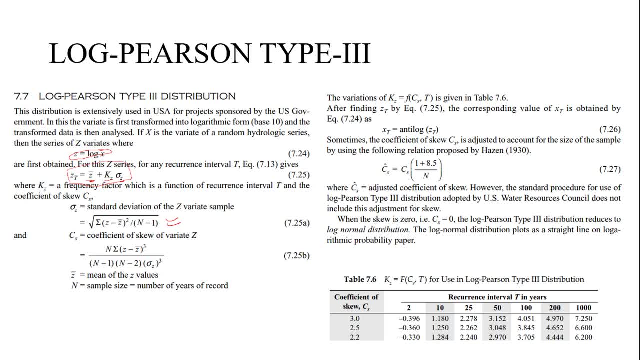 tables for the log p3. the tables require the value of the coefficient of skew, cs, and of course the return interval, that return interval and the cs. you can calculate the value of k and what is the cs value. cs is the coefficient of skew. this is given by n z minus z, bar q, n minus 1 and minus 2, sigma z, whole cube. 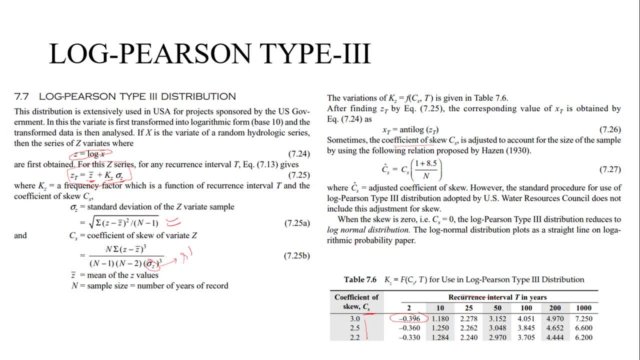 all these are standard terms. sigma z, standard deviation, and is the sample size, z is the, of course the discharge, z bar is the mean discharge in the log case. i think it's clear: once you get the zt, you can get the xt right. so now design flood. 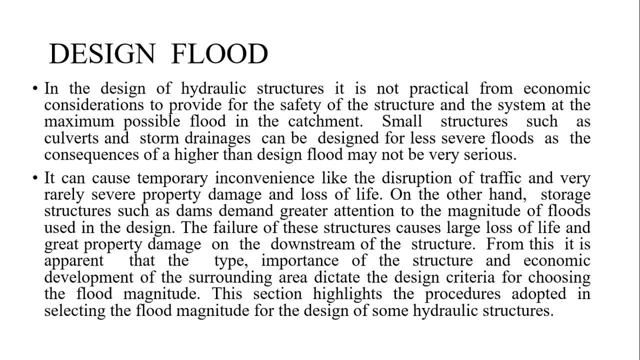 yeah, so the design flood. so we discussed in the beginning what is the design flood. whenever we are designing a hydraulic structure, we have to consider the safety of the structure. and for the safety of the structure we design it so that it lasts for a particular number of years. 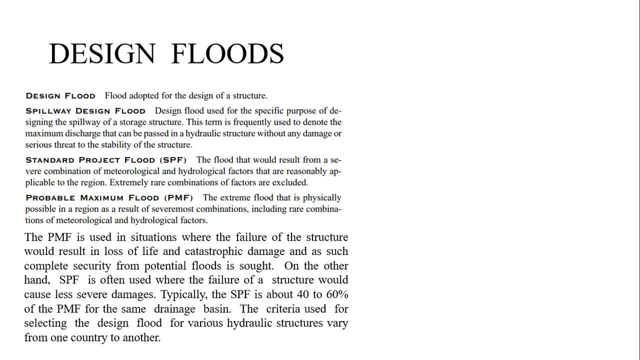 so there are number of definitions for the design flood. so spillway, design flood, it is used for the specific purpose of designing the spillway of structure storage structures. this is specifically for the spillways and there is a standard project flood and then there is a probable maximum flood. 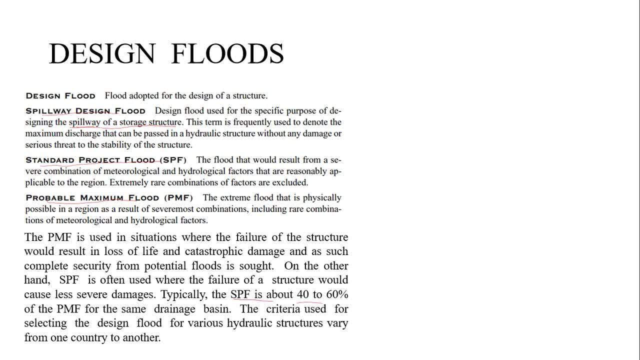 so mostly the standard project flood is about 40 to 60 percent of the probable maximum flood. so whenever we need more safety we go for the higher maximum flood value. so this is the, i think, highest problem maximum flood. this is extreme flood that is physically possible in region and this is severe. 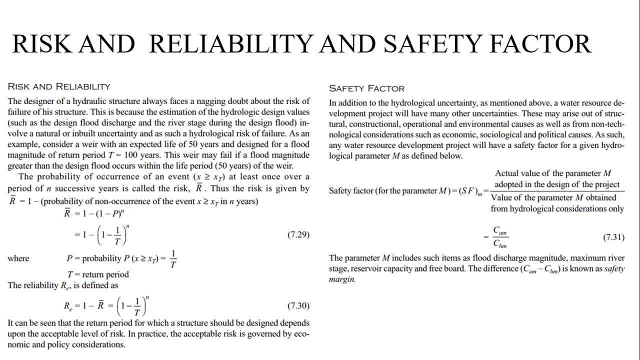 mode. so this is the extreme case for the floods. from the floods we have some factors like risk and reliability. it's a simple equations like: so, let's say, the probability of occurrence of an event at least once over a period of n successive years is called the risk right probability of occurrence of an even event occurring at least. 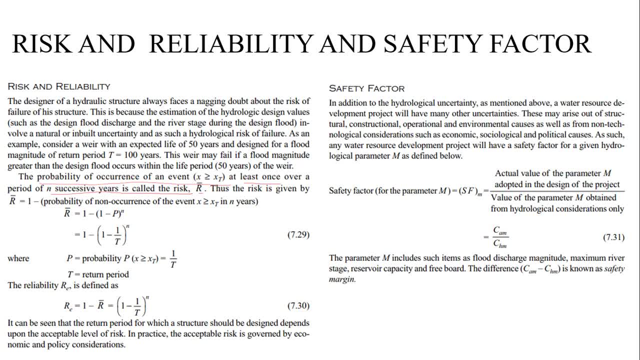 once over a period of n successive years, is the risk r. so risk is we had seen that formula. that risk is one minus. q raised power and so for the uh consecutive n years, if the flood is not occurring, this is called q is for n, and once in those n years the flood occurs, this is one minus. 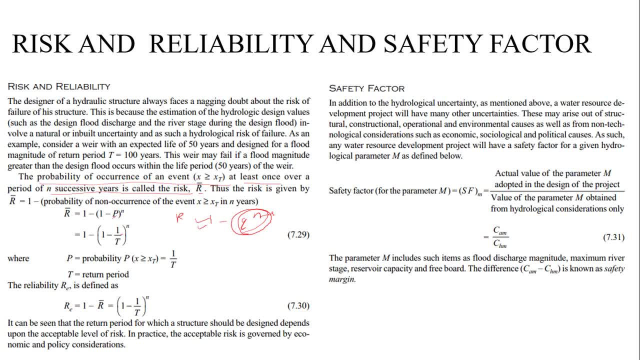 curious: power and and where p is one by t. so this is your risk factor, if you have the probability one by t and reliability is the. if you subtract this, this risk factor, from one, you get the reliability right and this is the safety factor. this i think you mostly apply in in many studies. so this is 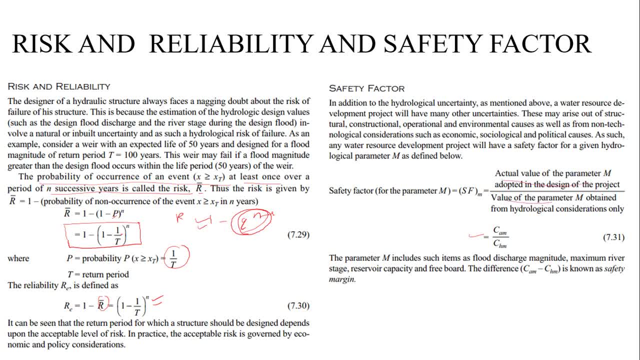 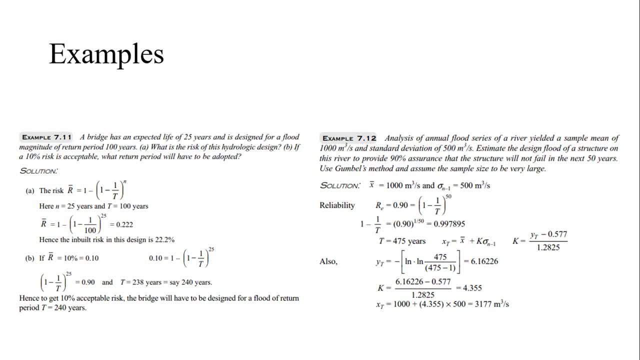 actual value of the parameter divided by the parameter obtained from hydrologic concentration. so this is the safety factor. so mostly we apply a higher safety factors. okay, so a simple a couple of examples to calculate the risk factor. so a bridge has an expected life of 25 years. this is expected life. 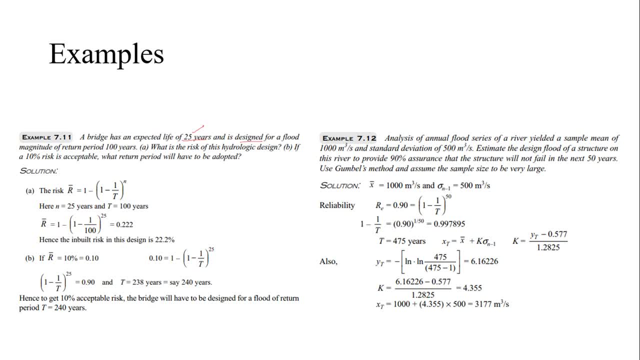 and it is designed full of for a flood. magnitude of return period: 100. so return period is given 100. so from this return period you can get the probability. once you have the probability, you can get the risk factor. this factor is zero point two, two, two. so the risk in this design is twenty. 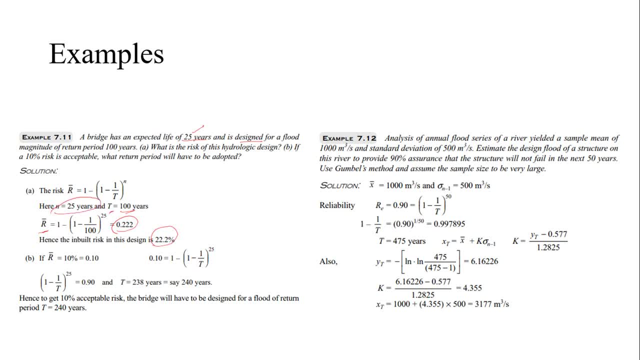 two percent. of course, n is 25 years. this similarly uh. if a ten percent risk is acceptable, what is the return period? so risk is given as ten percent. using this equation: zero point one. zero equals to one minus one minus one by t. from there you can calculate the return period this comes up with. 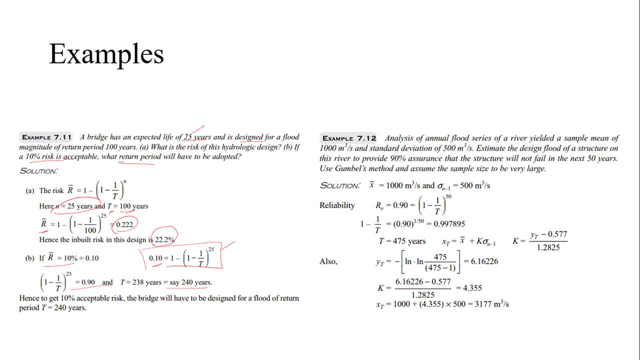 240 years. so risk is high. the written period is the expected life is less. if you go for lesser risk, your return period has to be higher. if return period is higher, that means your flood discharge will be higher. so you design for a higher flood discharge. as simple as that.